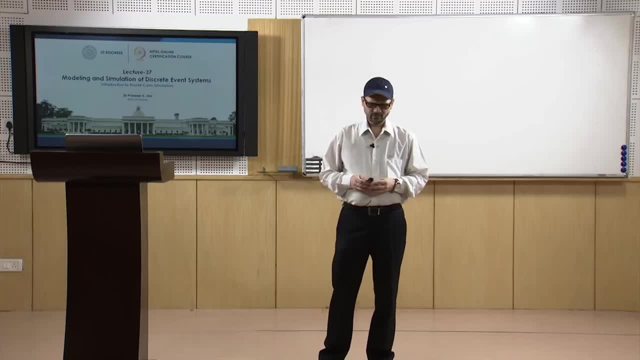 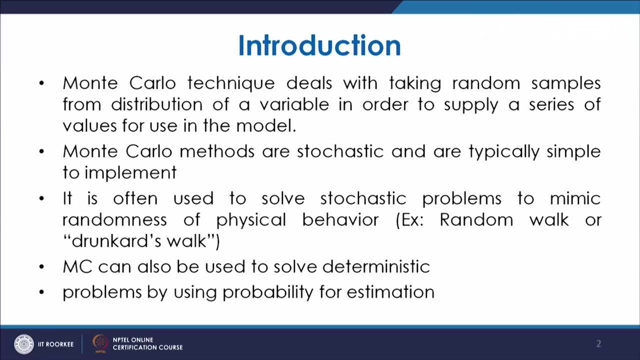 very difficult And in this what we do is we use the random numbers to basically model the process. So Monte Carlo technique: it deals with taking random samples from distribution of a variable in order to supply a series of values for use in the model. So, as we discussed that, in this we have to take the random numbers. 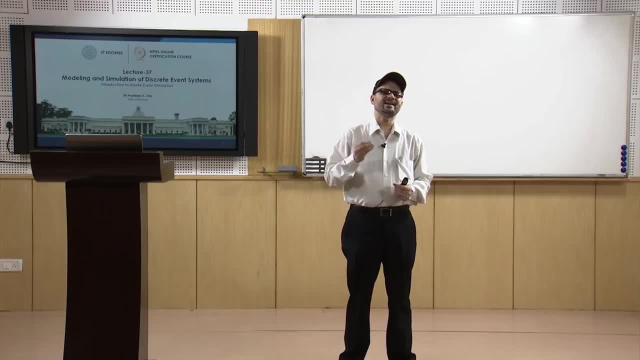 and these random numbers will be assigned. basically, there are methods depending upon the probability distribution or depending upon the chances, which have been told to you or which is basically clear in the question. So, based on that, you assign those values against certain random numbers and these random numbers are basically uniformly distributed. 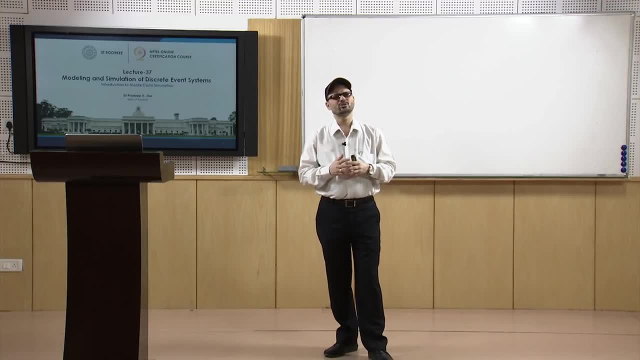 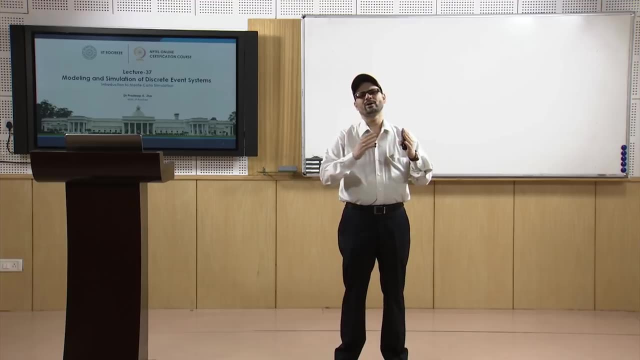 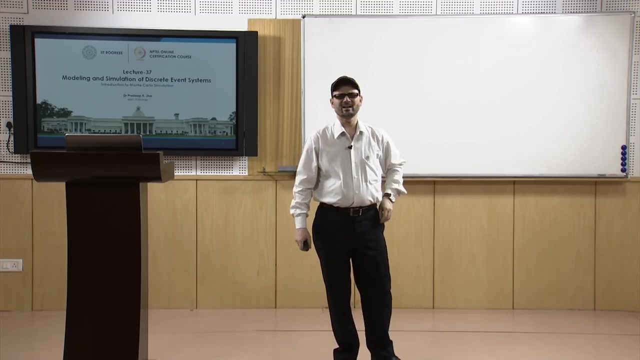 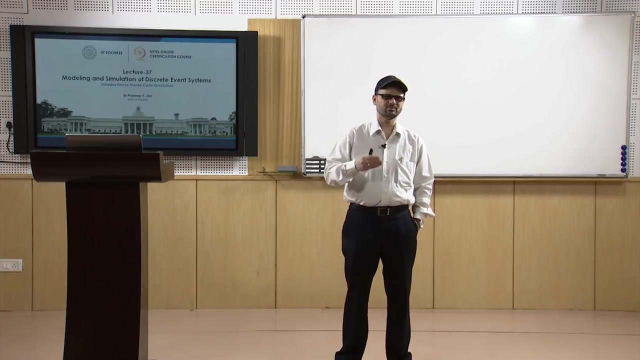 So you can have the generation of these uniformly distributed random numbers between some quantities, like between, suppose, 1 to 100, 0 to 99, or you can have 0 to 1. ok, So we have the studies, the algorithm or the methods of generating these random numbers in the chapter random. 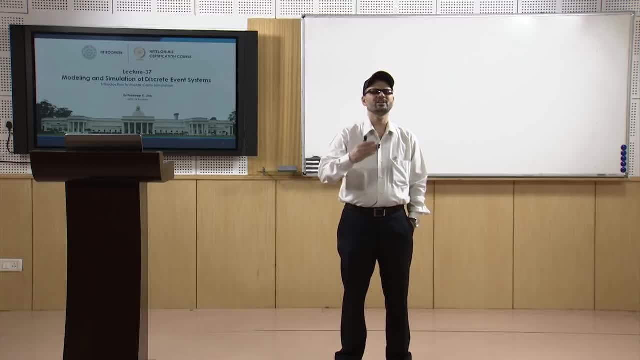 number generation. So in that random number generation we studied the methods like linear congruential generator, we studied the method that is mixed congruential generator. Then also we studied about the method that was random variate generation. So where we had 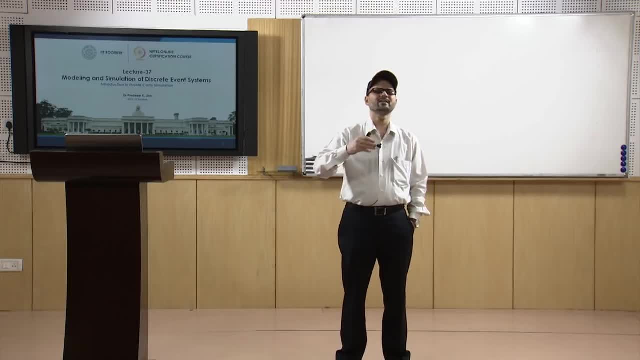 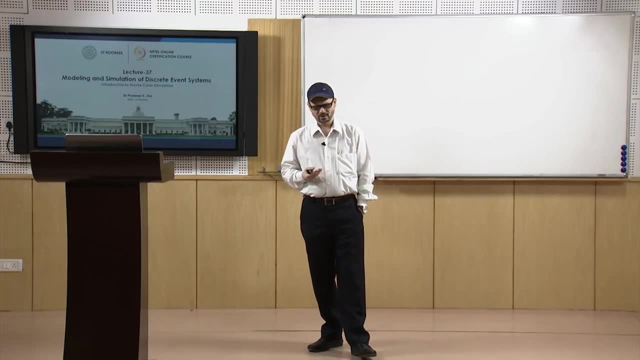 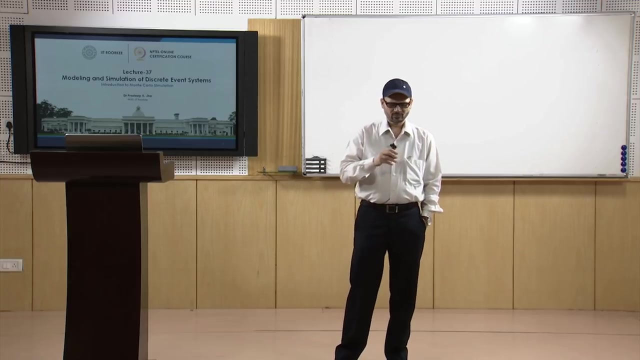 to generate these random numbers according to certain distribution function. So we use the cumulative distribution function for certain typical distribution function and then, by using the inverse transform, we are generating the random variate. So these random variates are there, random numbers are there and these random numbers. 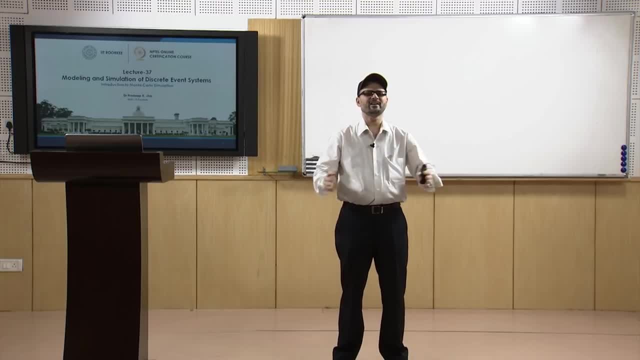 are picked up, I mean, anyway they are generated- then they are basically uniformly generated, So the probability of any random number into that domain is equal. so when they are used, and then they are further used for predicting the system performance. So let us now go further. First one, which is それ, ranks agricultural. 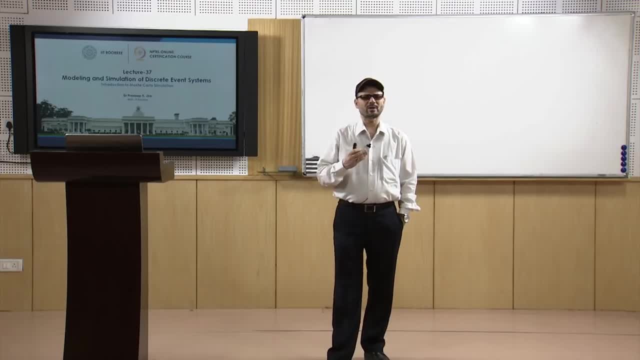 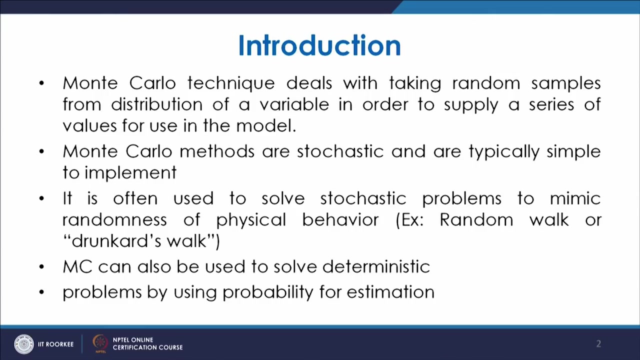 So they are stochastic and they are simple to implement and it is often used to solve stochastic problems, to mimic randomness of physical behavior. So just you can have the understanding what is random like there will be random walk by a drunkard person who can put his foot any at any place and he can go in any direction. 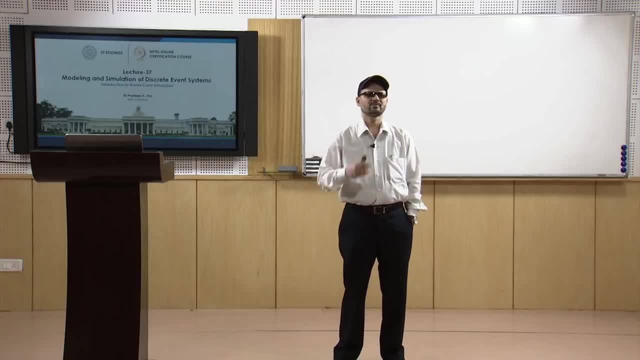 So that is like the example of randomness. We can even solve some deterministic problems by using the probability for estimation. So this Monte Carlo method can be used for that purpose. we will have an example and we will see that how we can find the variables. 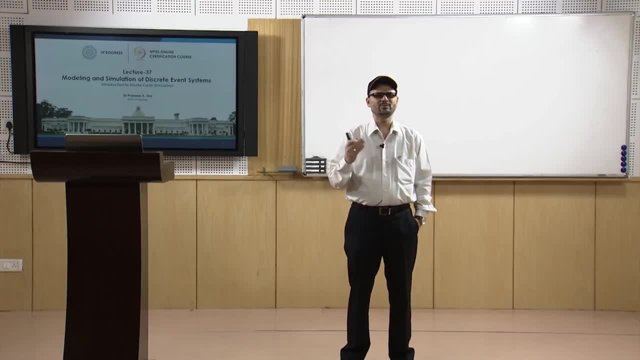 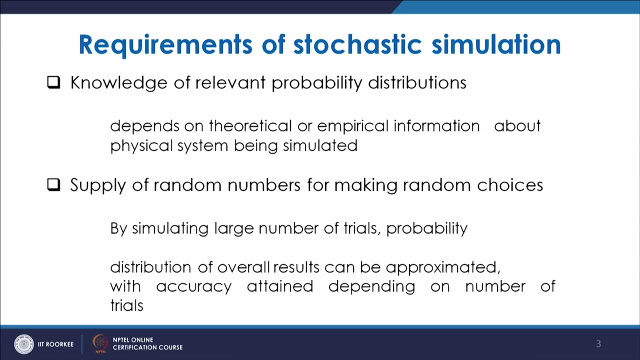 So value of certain quantity which is determined, and how can we find by the random means, Monte Carlo method? So what we need to go ahead to know about the Monte Carlo simulation or stochastic simulation, So you should have the knowledge of relevant probability distribution. 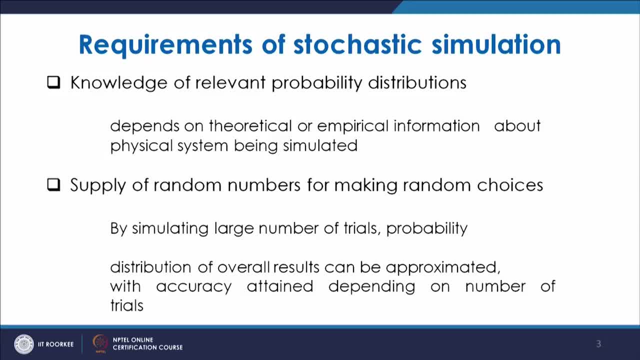 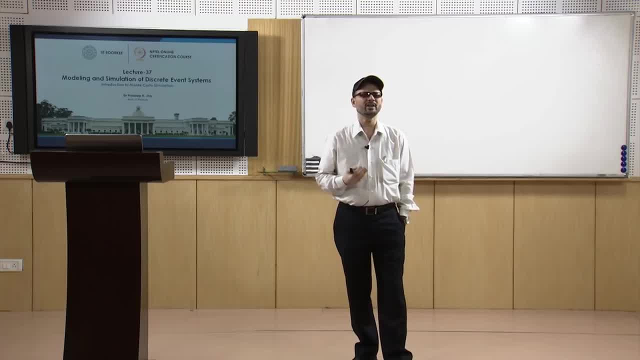 So that you can generate the random numbers, if required for particular distribution you should have. So this is the idea that how this distribution behaves. if you have to predict any quantity, then how to predict it, how, with what kind of distribution it will be matching. 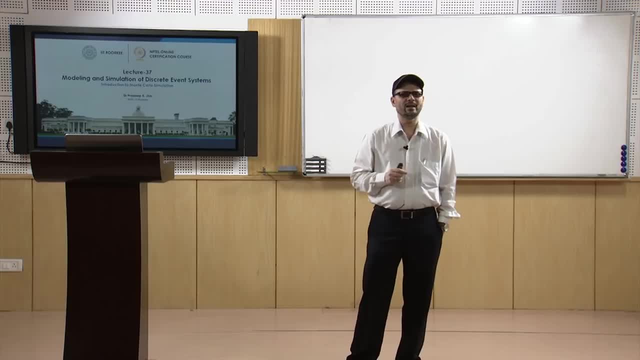 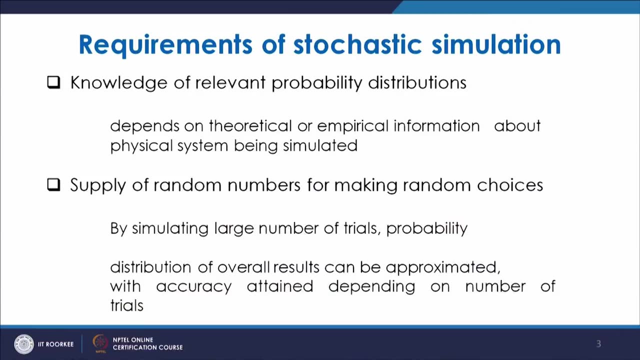 So that, basically, you must know that, So you must have the information about the theoretical distribution- I mean distribution or empirical distribution- And about the system. So that is the idea, So the system for which you are going to study now: supply of random numbers, of, for 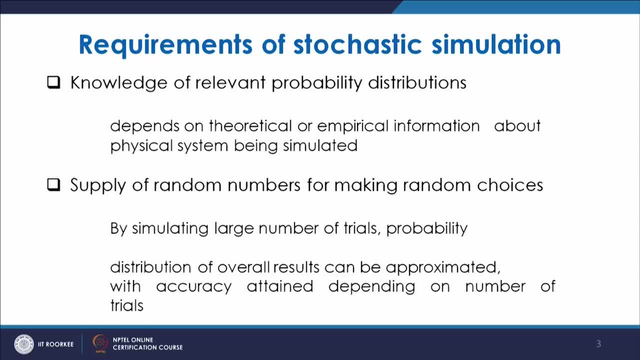 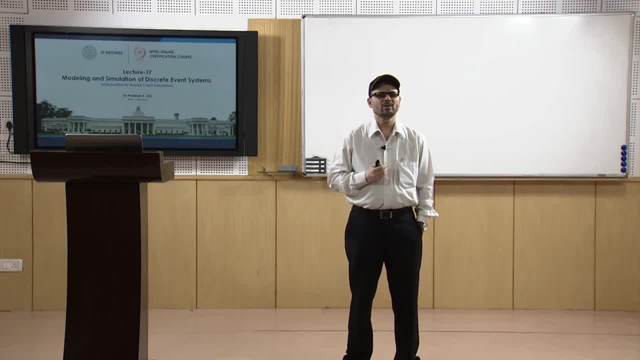 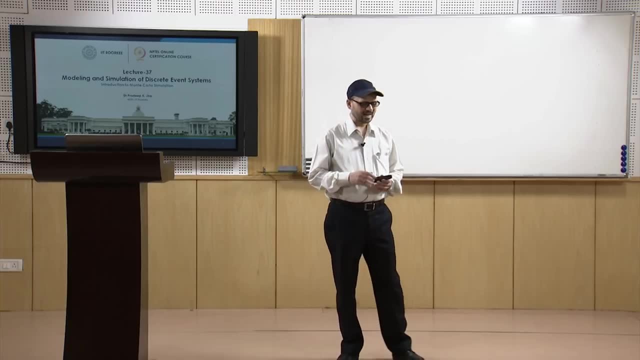 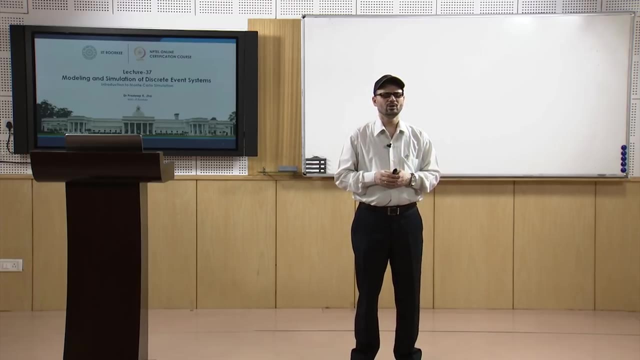 making random choices. So what? there are many methods and you can simulate large number of trials and probability. So that way the accuracy will be more and more So as we do more and more number of iterations in that, So we are coming closer to the actual value. 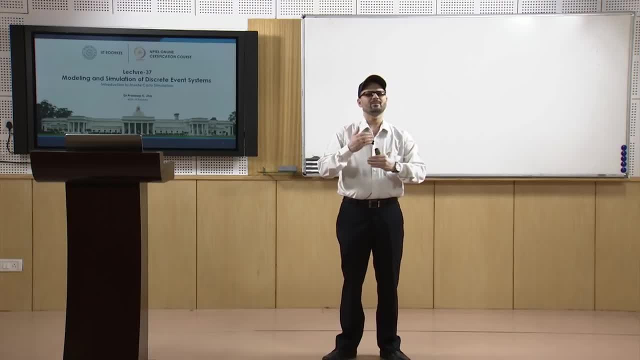 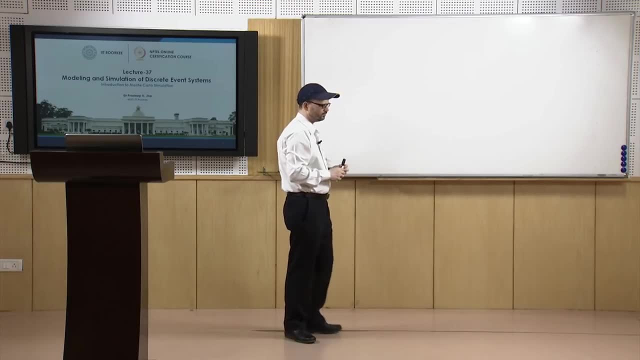 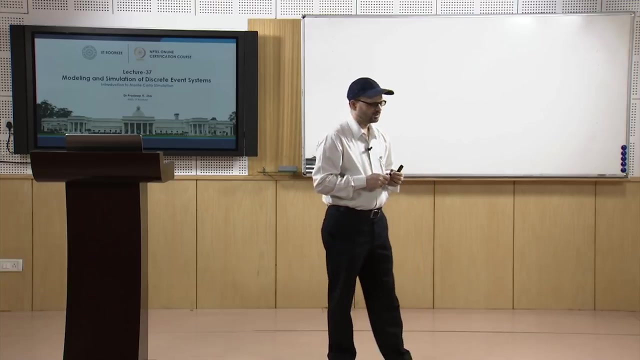 So we can see how this random number works. what happens in that? Now let us see how. what is the process in that So many a times you come across the probability of occurrences? suppose you are dealing with the- you know- lead time or you are dealing with the arrival time. 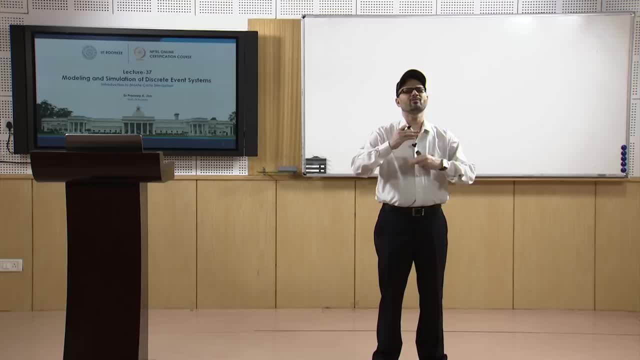 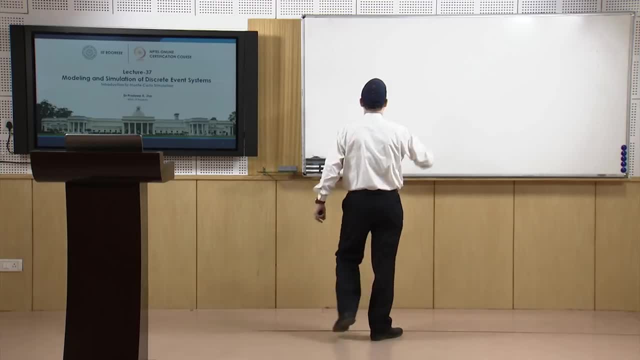 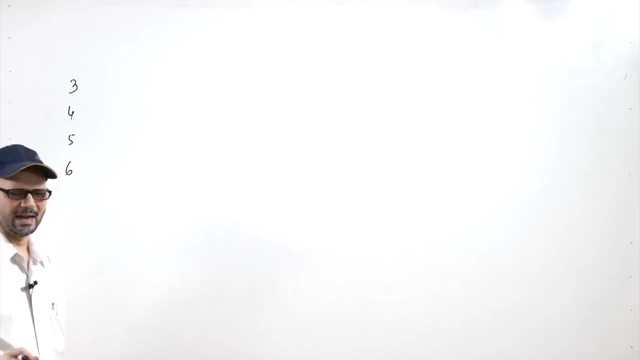 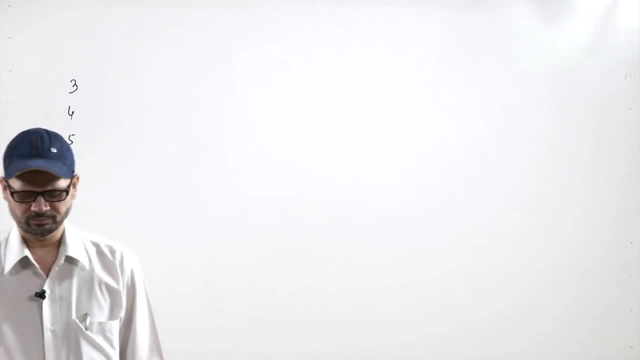 So you are dealing with the arrival time. So you are dealing with the arrival time. So you are dealing with the arrival time. Suppose, 5 minute of interval. it was seen that either there will be 3 number of arrivals, either 4, either 5 or 6 number of arrivals will be there and it is said that it has the 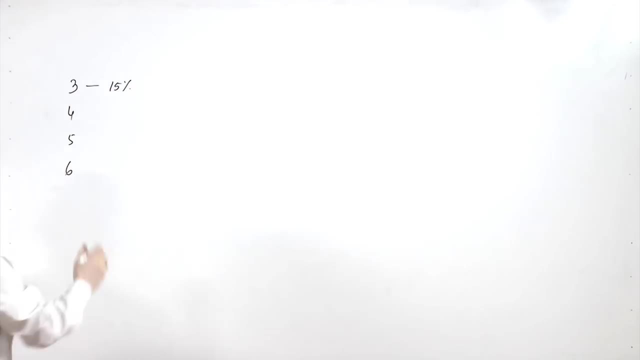 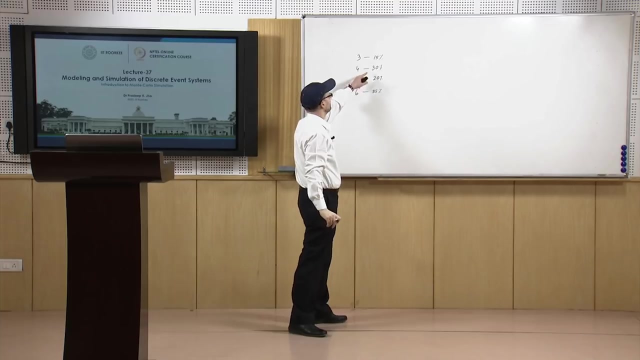 probability of, suppose, 15 percent, it has the probability of 30 percent, it has the probability of 20 percent and this has again the probability of 35 percent, suppose. So this is told to you. So it is 35 plus 20.. So it will be 45 plus 20, 65 and 35 hundred. 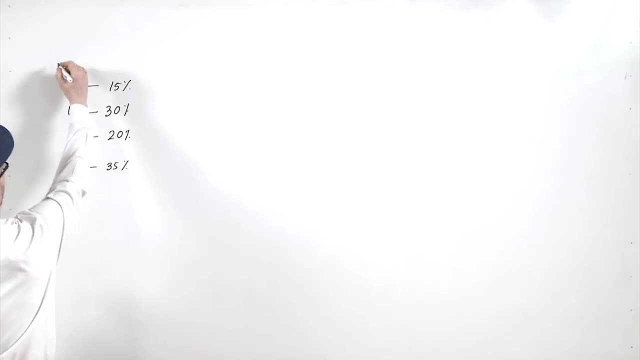 percent. Now, if they are telling that, suppose this is the arrival rate in it, in suppose in 5 minutes, and this is the probability. Now, if suppose you have to see, you have to do the random. 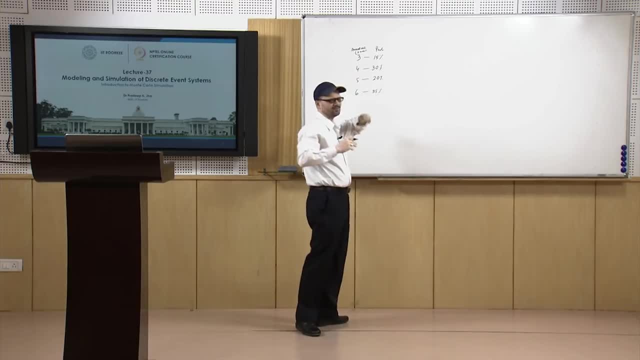 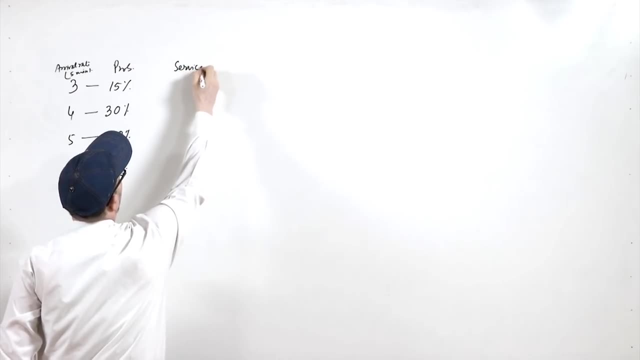 the sampling and then there is arrival of the customer. simply you have the service rate. So simply service. also, if the service is done, service rate is there in again in 5 minutes and if they, it is seen that there are 4 services done, there are 5 services done and 6 services. 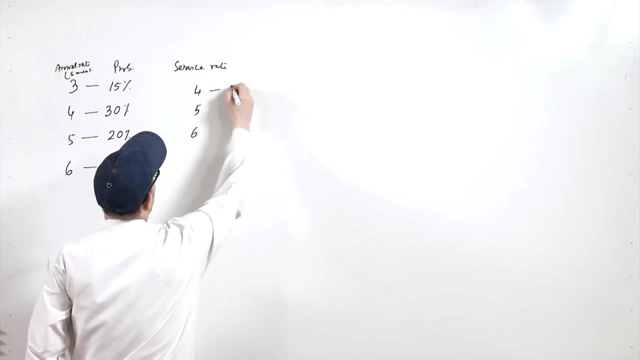 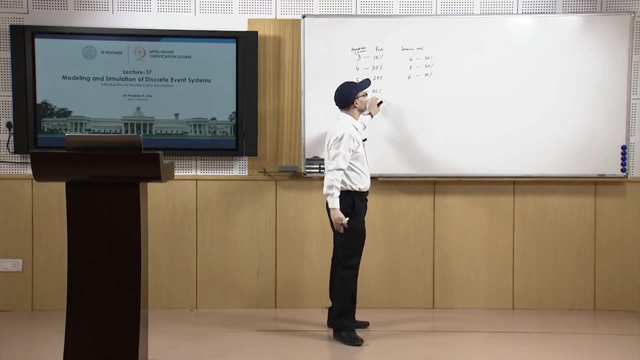 done and they have the probability of say, this is 30 percent, this is 40 percent and this is 30 percent. So what we do is that. but because they are not following any typical distribution, we know that after looking at the data, we came to this conclusion. we have concluded that 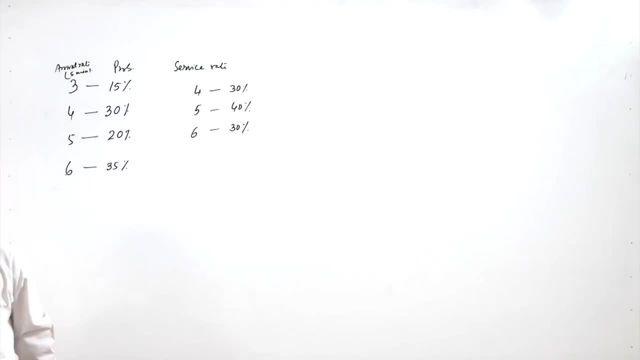 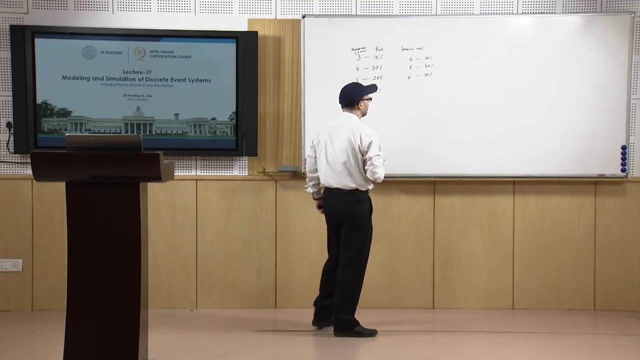 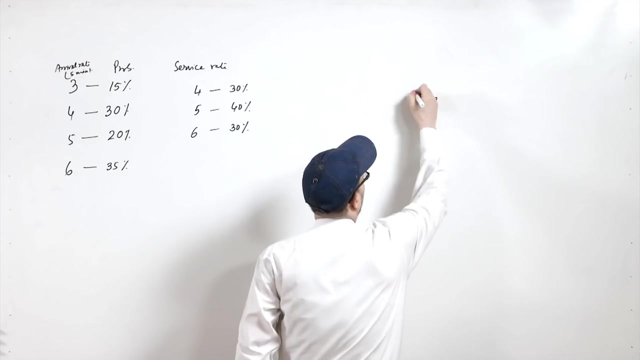 out of these 4. these are the respective probabilities. Now, how to get the help from the random numbers. So what we do here in this that normally, normally the process, is that you have the frequency, So you will have the number. So 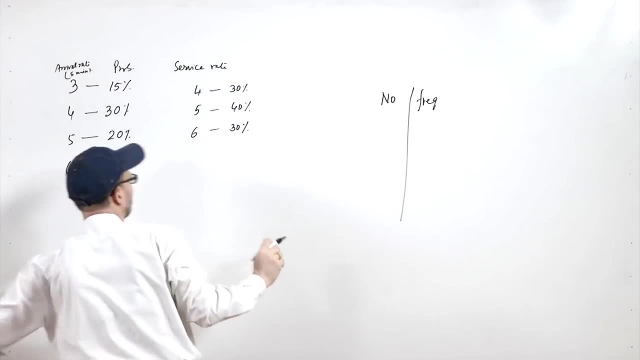 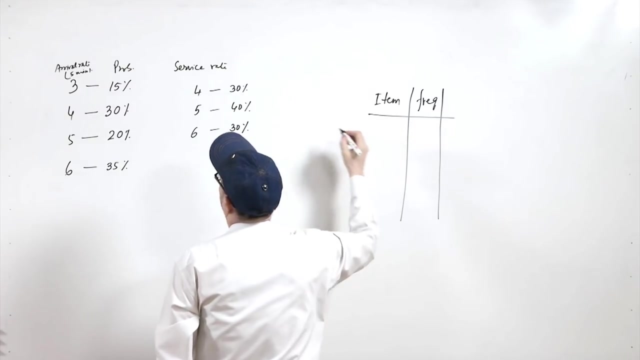 whatever is there, arrival rate or item is there? basically, this is not the number, this is suppose. whatever item is there, whatever quantity you are going to, you know predict and its frequency. So, as we know that, if it is, you know arrival rate. So arrival rate. 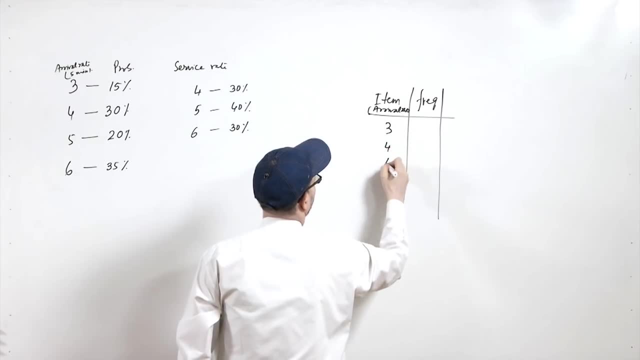 we know that you have 3, 4, 5 and 6. Now in this, as we know, the frequency is 15, 30, 20 and 35. So what we do is we find the cumulative frequency. So once we find the cumulative frequency, So cumulative frequency will be here. it is. 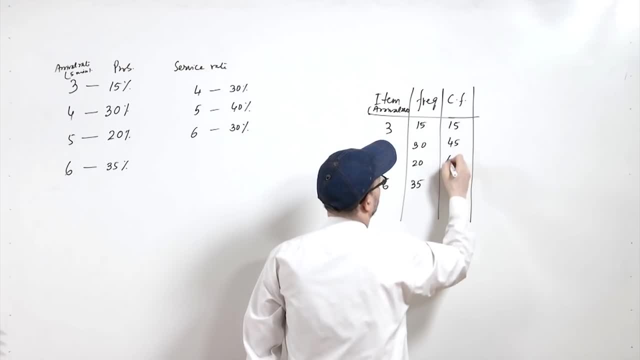 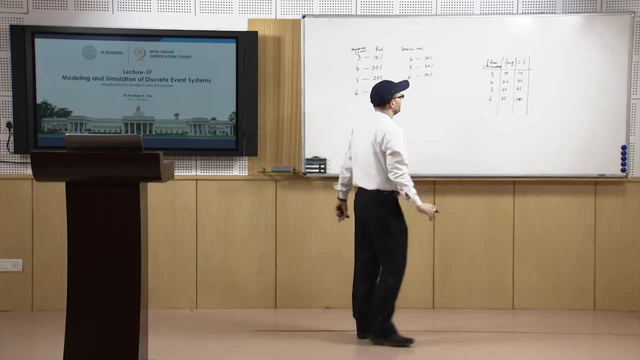 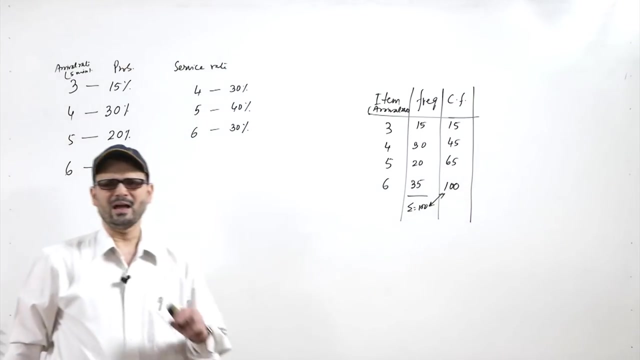 15, this will be 45, this will be 65 and this will be 100.. So, ultimately, the cumulative frequency comes here, because this is total is 100. So you are matching it. Now you have, if you have, the uniformly distributed random numbers between the number of items. 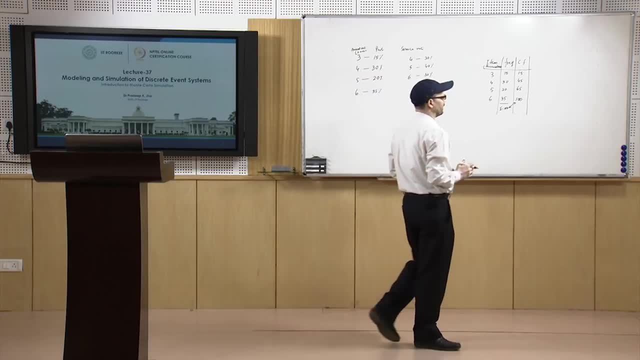 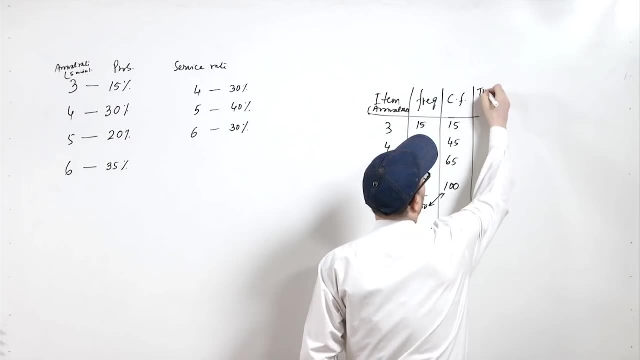 between 0 to 100. So, excluding 100, because we will take the 2 digit number suppose. So for a 2 digit number, 2 digit random number we have to assign. So what we do here is, as we know, that this is the uniformly distributed random number. So the probability of the 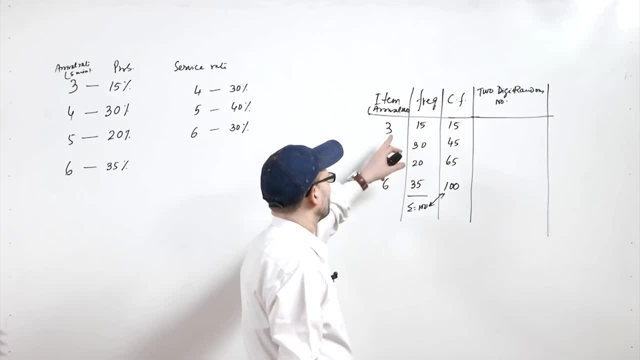 picking of any number is same. Now what we see? that if we are having this 3, it must have 15 percent of the probability. So basically, if we start the number with 00. So up to 14 it will go. So we randomly 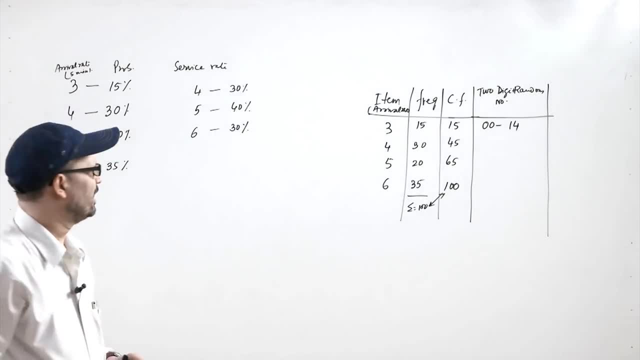 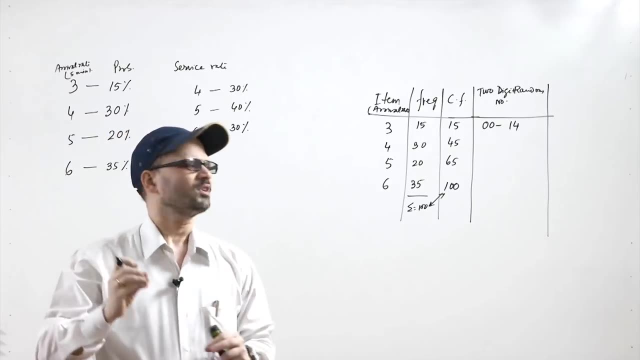 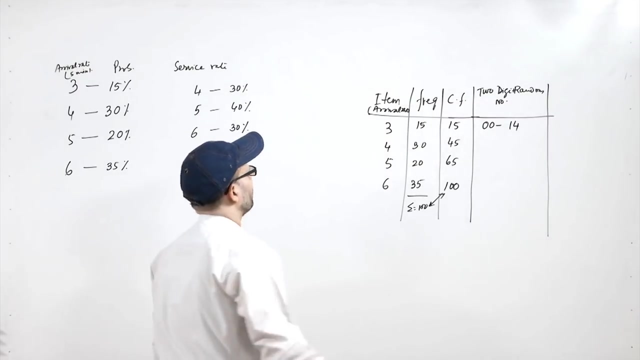 pick any number and if that number will be from 00 to 0 to 1- 4, then we will assume that this time we have to pick, So we have to take the arrival rate as 3.. So basically that arrival rate will define. 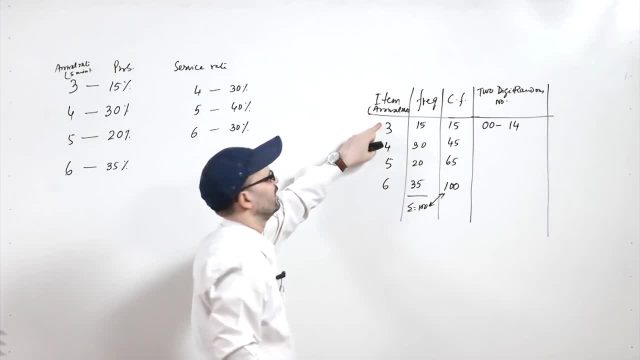 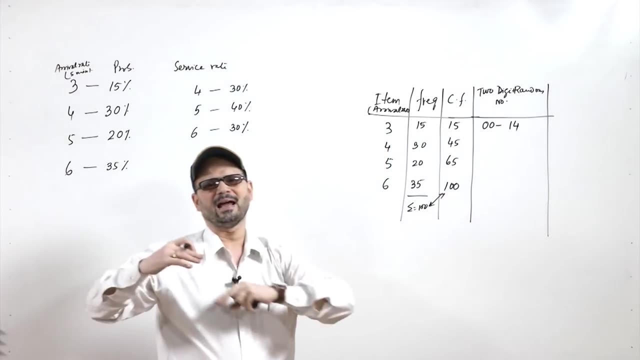 the entire arrival time basically. So from here you will find the entire arrival time. So let us see for this. we have done So anyway. if this is there, then we can have the entire arrival time. So basically, we are going to estimate the entire arrival time. 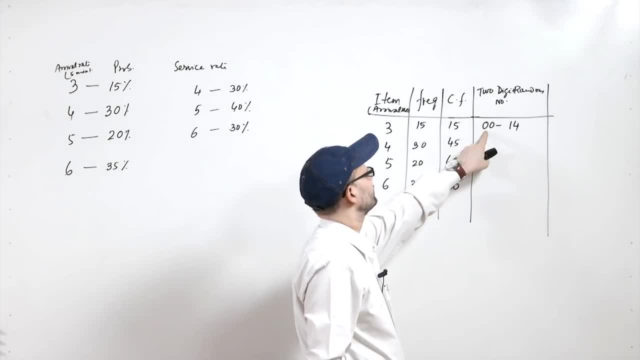 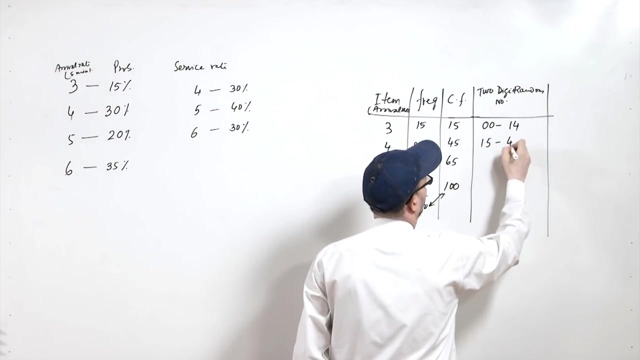 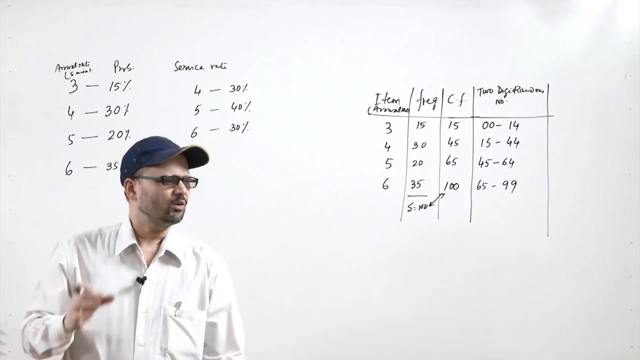 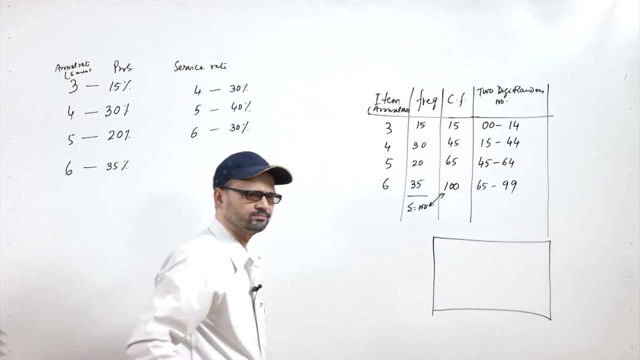 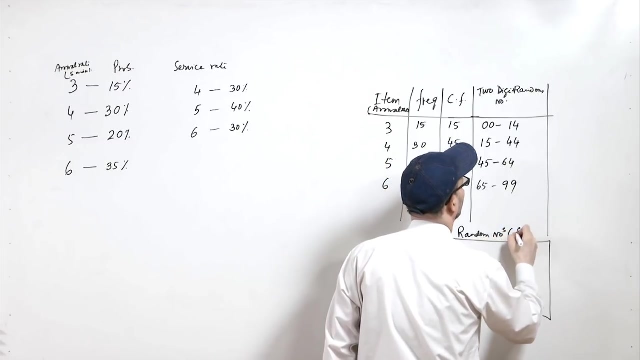 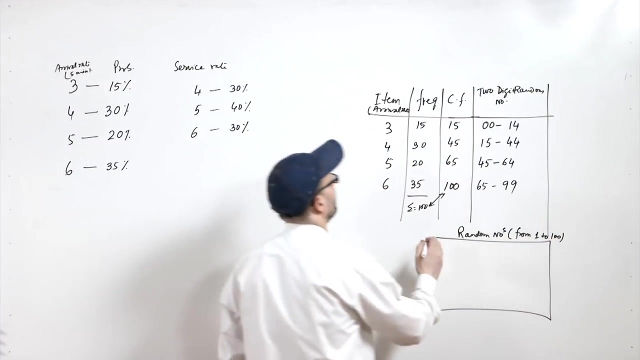 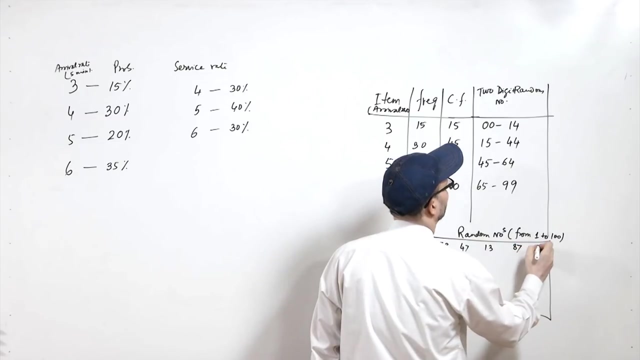 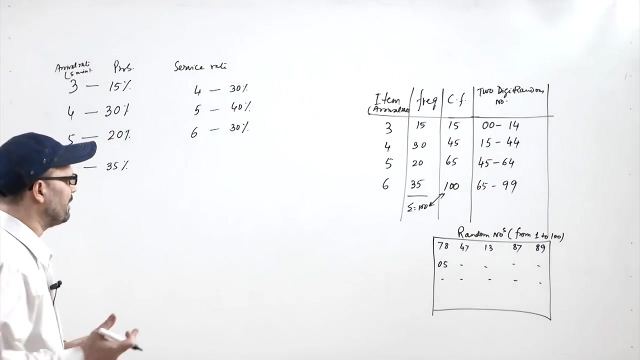 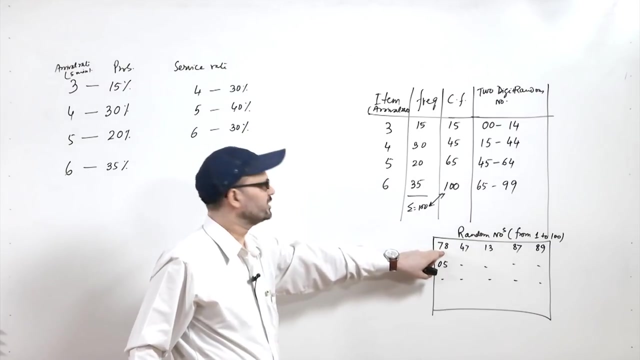 from this. So this way you can have the random numbers uniformly distributed, random numbers generation. Then what will happen? you will start from here. you will take 78.. So in the first iteration, if you take the first number as 78, this 78, you will see that it comes where. So it is. 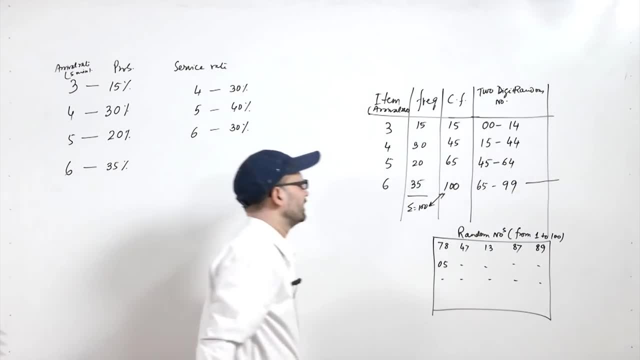 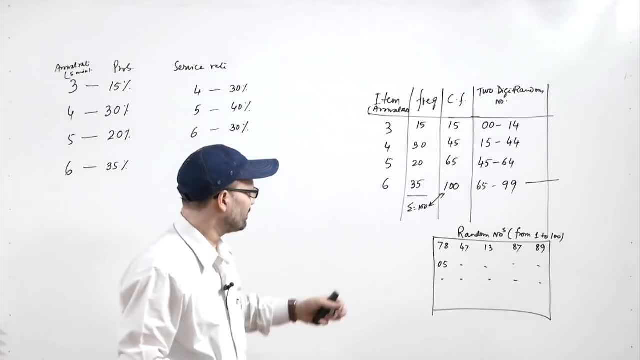 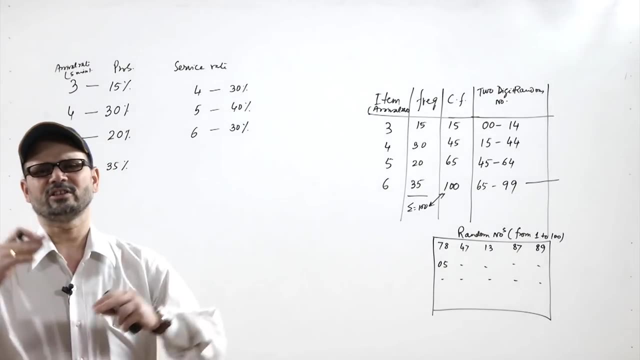 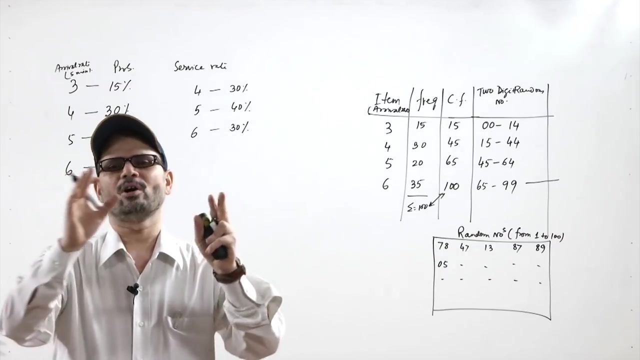 these numbers will be taken in a sequence manner and these numbers are basically uniformly distributed. uniformly distributed means if these numbers are plotted against each other. so if you have these numbers and then you generate another random number, ah, and then you plot them, then you will see that they are uniformly distributed in the domain. so 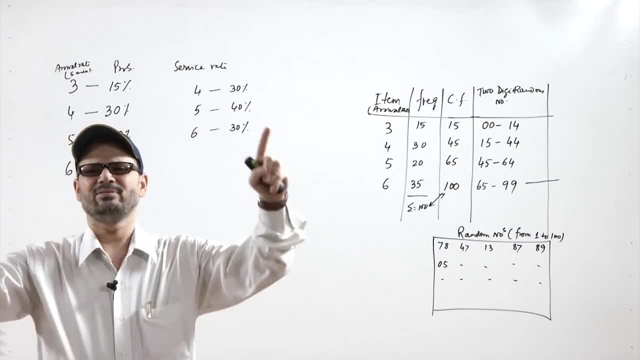 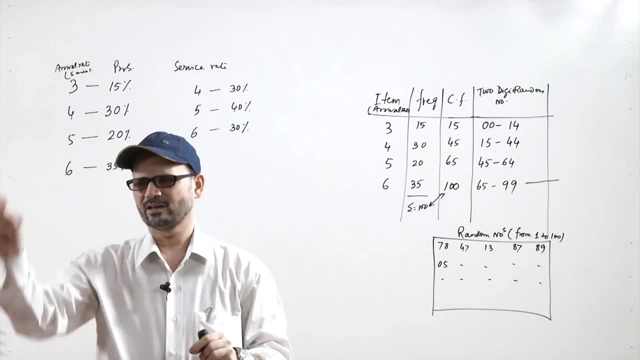 0 to 100 on the x and 0 to 100 on the y. so you will have the uniform distribution of the number in the whole rectangular domain, or square domain of 0 to 100 and 0 to 100 here. so similarly, if suppose here it is, 4 is 30. 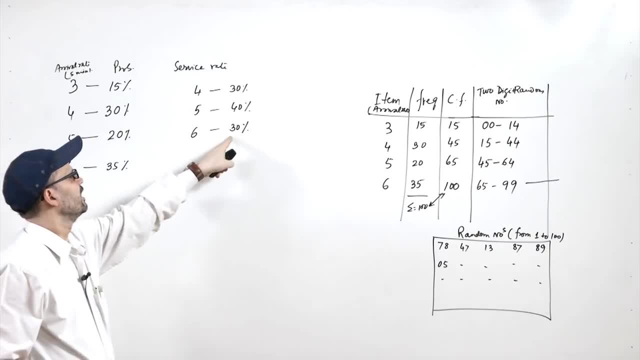 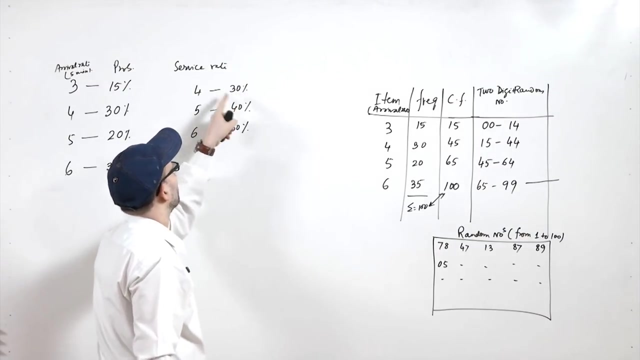 percent, 5 is 40 percent and 6 is service rate. is that is 30 service time? basically, it will be so if the service time is 4 minutes or 5 minutes or 6 minutes in that case. so that will be so. 0, 0 to 29 will be required for this case. ah, so that if that number is 0 to 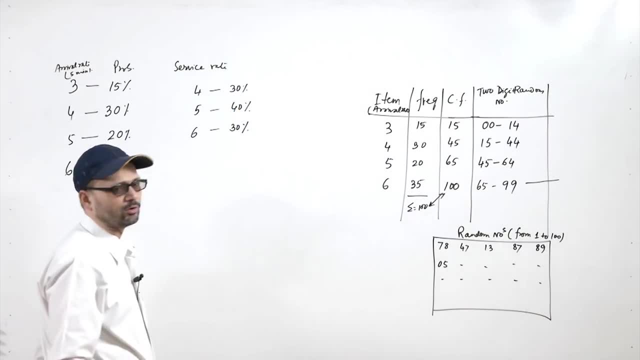 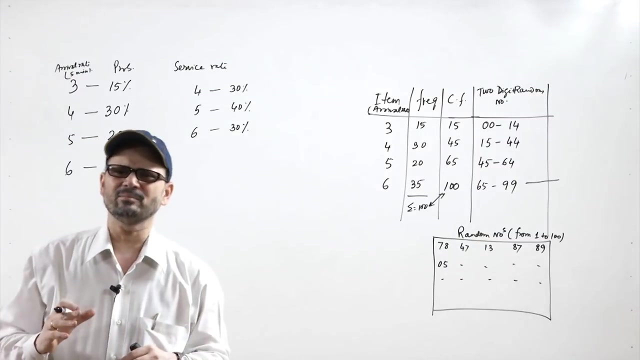 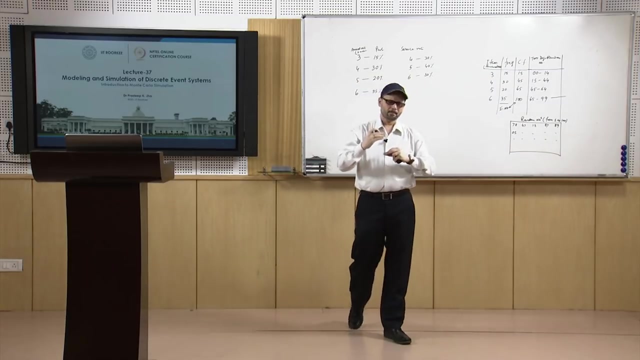 100, that will be basically for this 4. similarly you have the ah from 30 to ah. 69 will be for 5 and again 70 to 99 will be for 6. so this way we assign these random numbers and we try to get- i mean every time, whenever we require the ah values of those parameters whose ah. 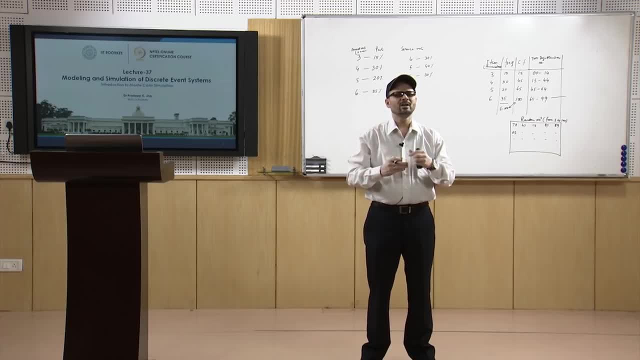 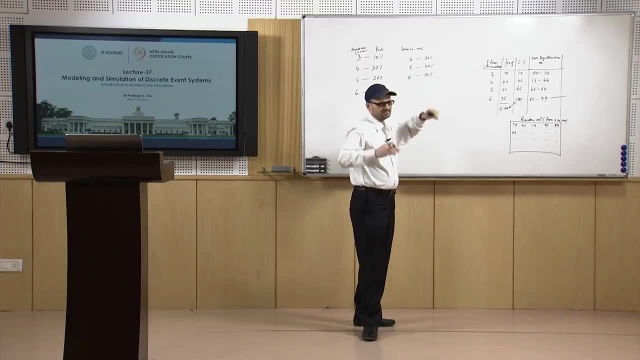 ah. So whose outcome is not known, about whom we have to have the you know chance. we have to know that. what will be the next then, taking the random number sample from that generated sample. you can have it now. you can have the generated number also, or variate from a particular. 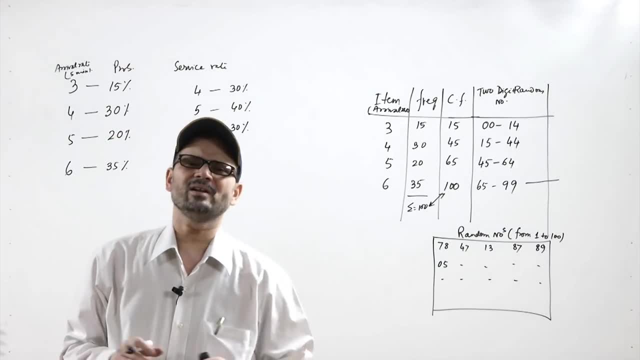 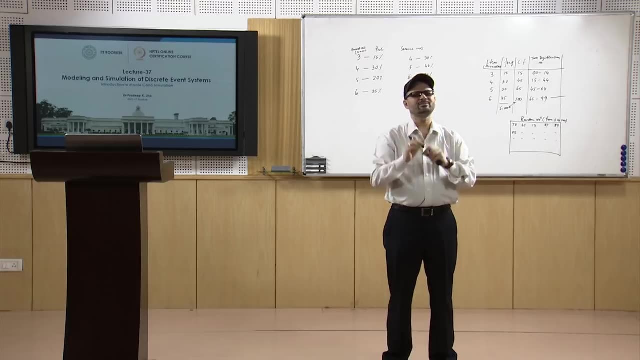 distribution also and otherwise. in normal excel ah software of microsoft you have the random function. So you simply have the random random function. it will give you the the uniformly distributed number, So you can generate any ah random number uniformly distributed between ah two domains. 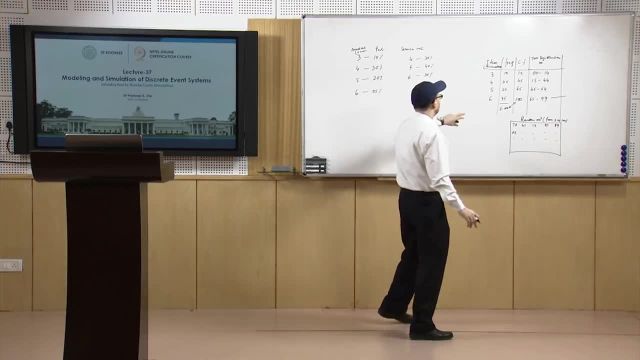 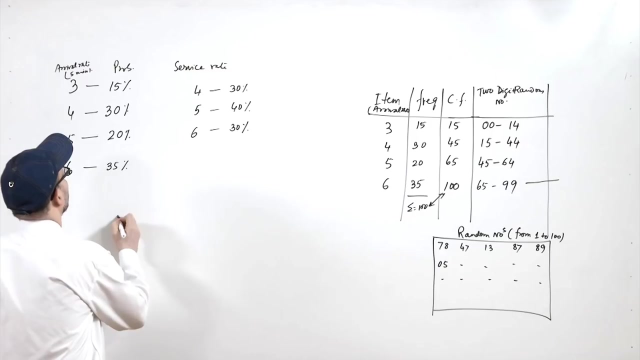 So we will try to see that. how can we? so let us, ah, we will discuss that. how can we calculate certain deterministic quantities, like suppose we have to compute the value of pi. So suppose we have to compute the value of pi by random number. 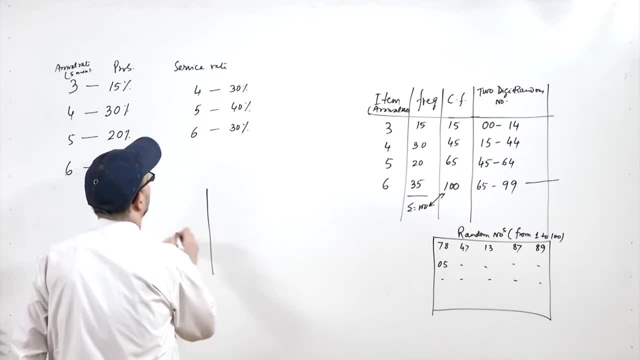 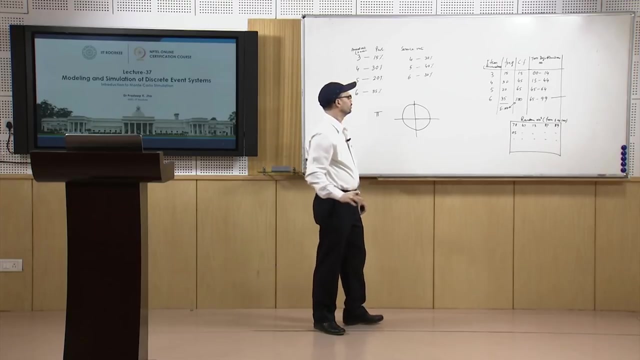 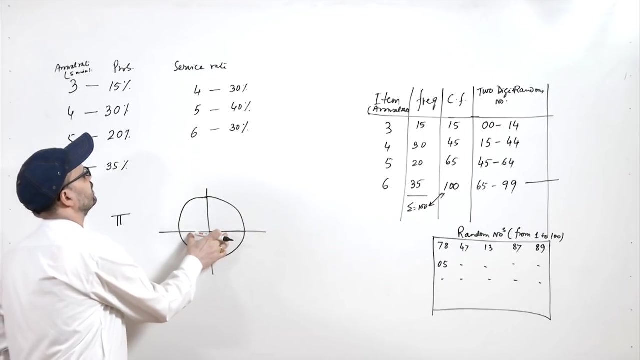 So what we see is that, ah, you see, ah, you know that there is a circle and if it is ah, diameter is 1, or if it is radius is 1, then the radius, the area of the circle, will be pi. So if we know, or if the, if the this ah value, if the diameter of this circle is 2, so if 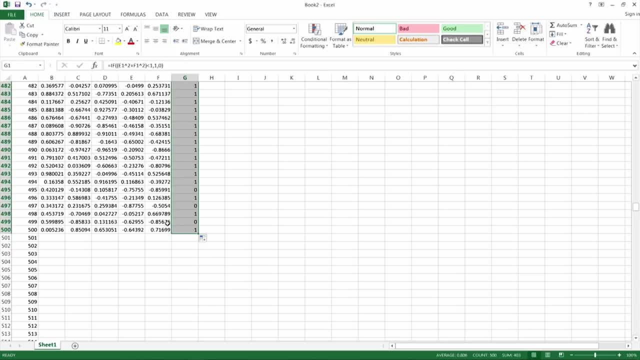 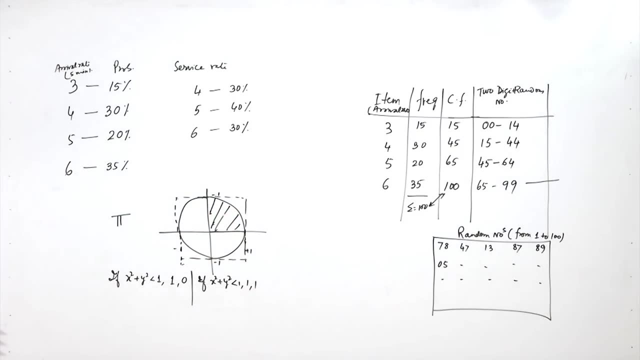 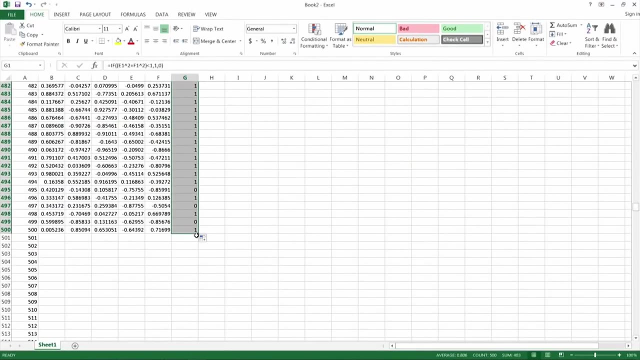 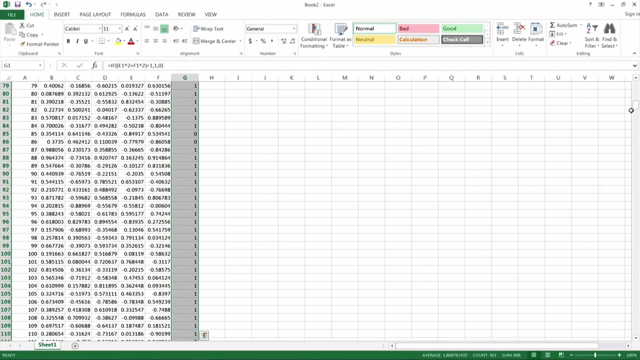 So it is writing 0 here. So where, wherever this point is going outside this domain, outside this domain, so that points are taken as 0, and then so there are 500 points. If you take the summation of these points, this point is summed out to be, let us say, 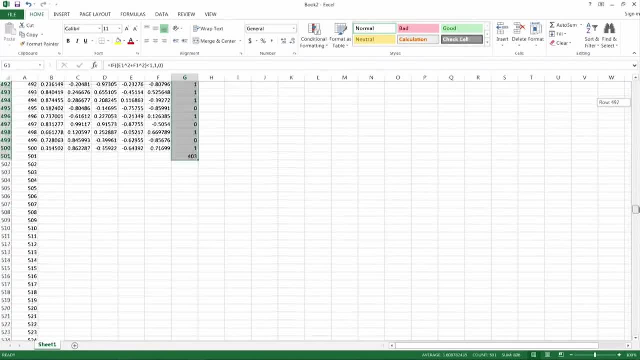 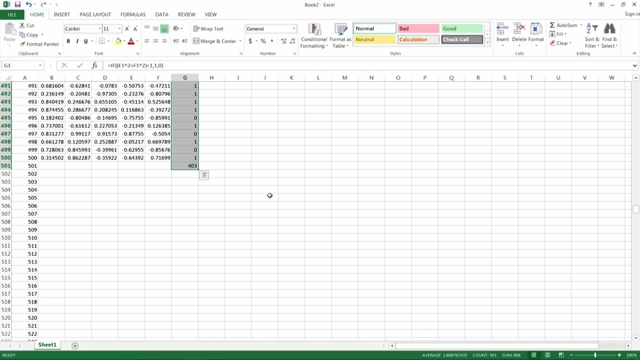 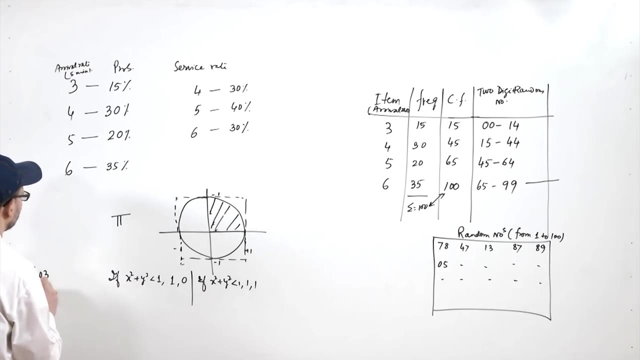 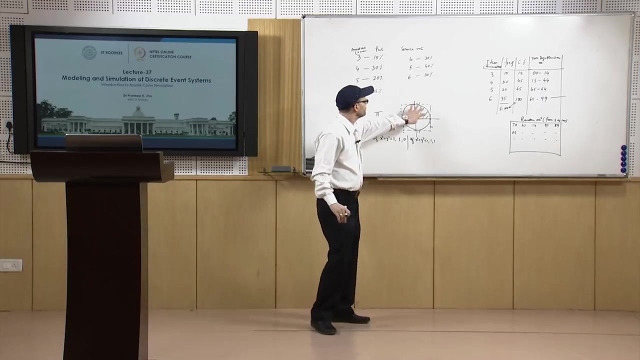 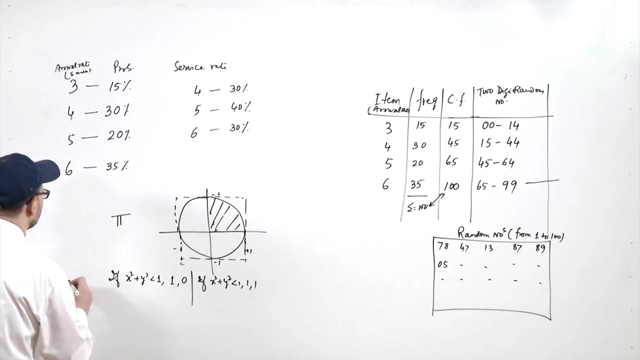 how much? this is 403.. So there are total 403 ones out of 500.. So out of 500 you have 403 points which are falling inside this. So basically it is coming out to be 0.8806.. So for only, 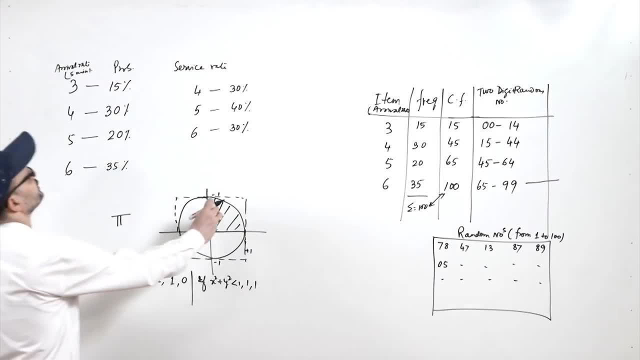 for 500 attritions and because this is the pi by 4 region, So for getting the whole pi value you will have to multiply it by 4.. So 0.806 multiplied by 4. So it will be 3.8806.. 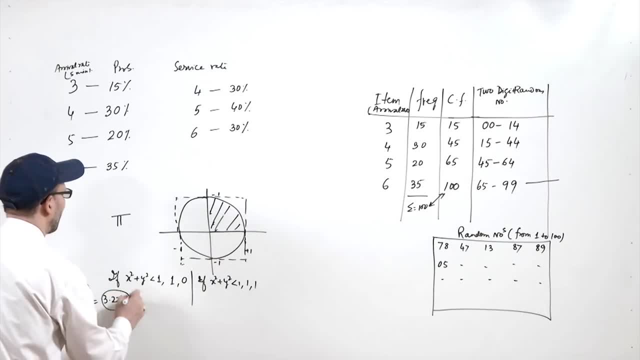 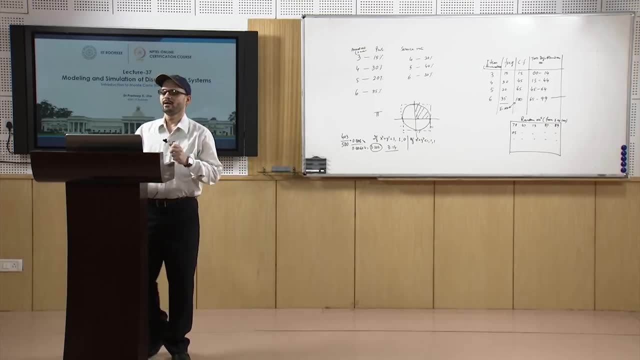 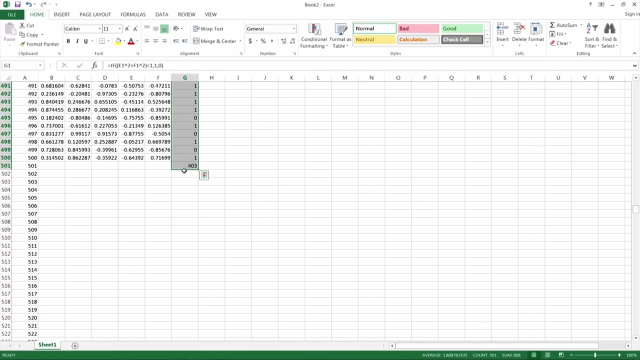 Whereas the actual value is 3.14.. Now why this difference is? Now, this difference is because we are doing only for the 500 cases. Now, if we do for more number of cases, if we do for 10000 number of cases, in those that case it will be closer and closer that we. 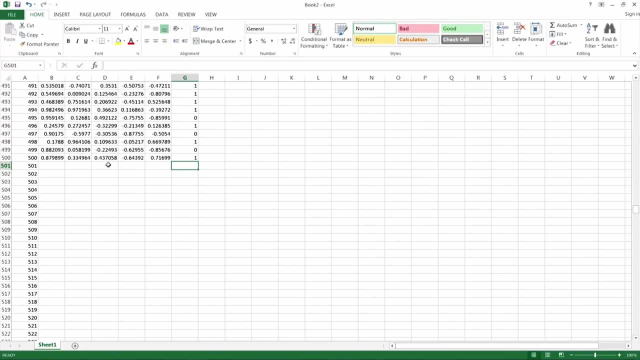 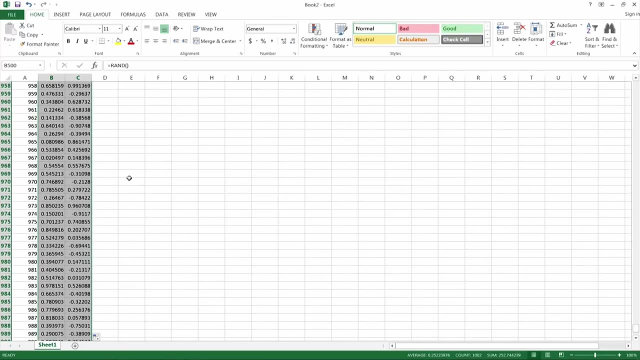 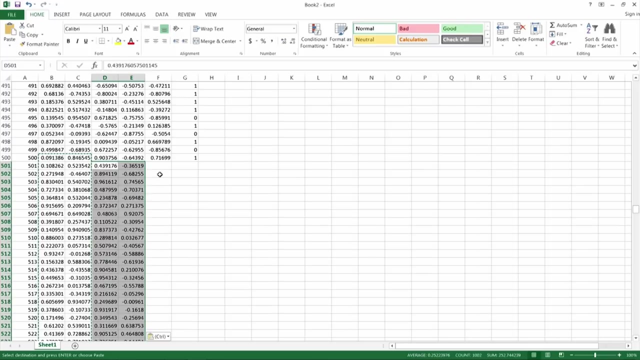 can check, Because we are generating another stream of numbers from 500 onwards and go say up to whatever we had decided earlier, up to 1000. So again, we are copying it and we will be pasting it, So we can again paste it. So we can, we have pasted them, So we have pasted. 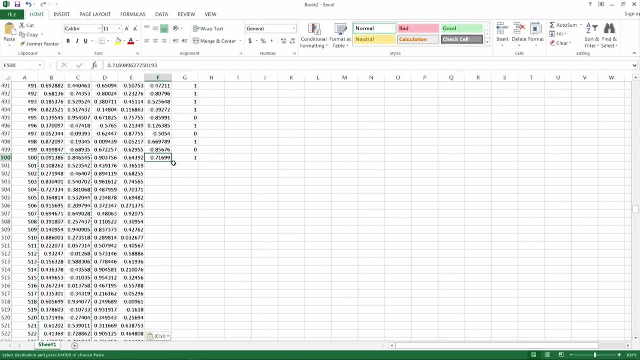 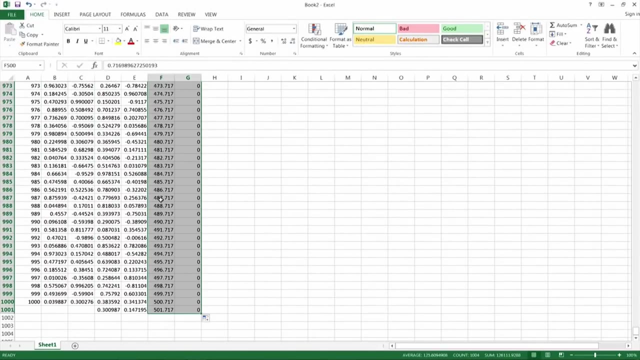 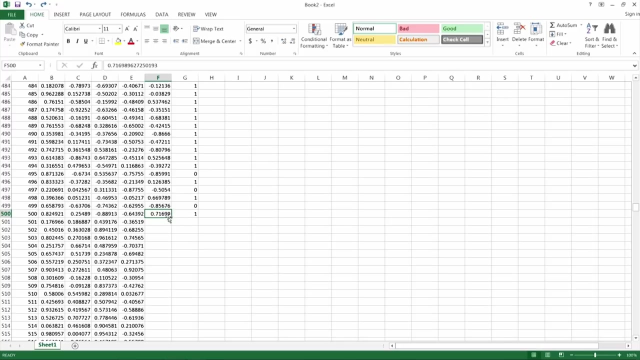 especially, and then we have further. we will have the condition So we can further drag them also. So if we drag them for 1000 now, in this case, now it has taken somewhat different way. So in this case you have to see that how these values are coming. anyway, 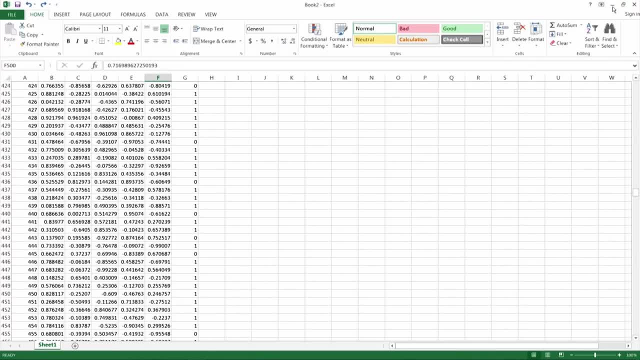 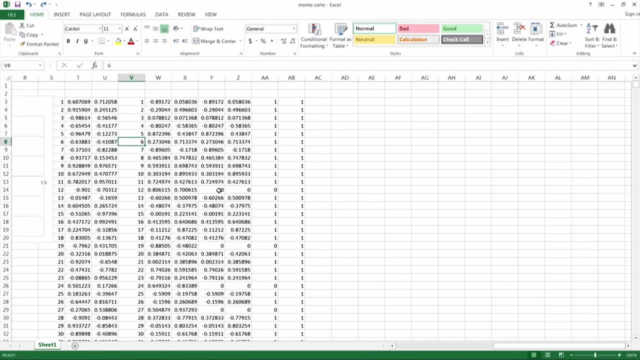 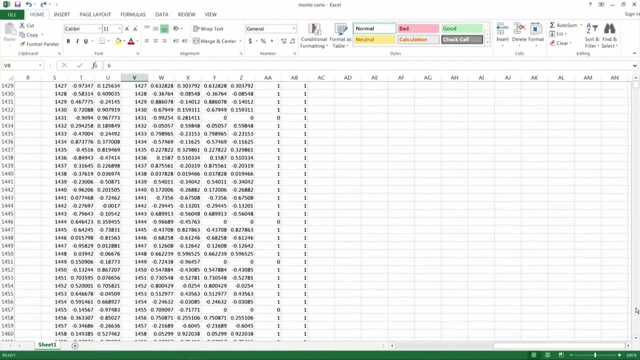 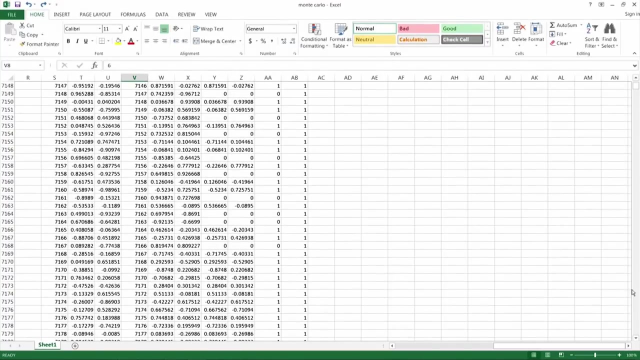 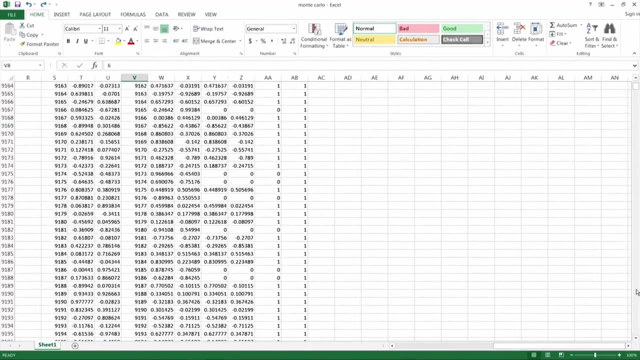 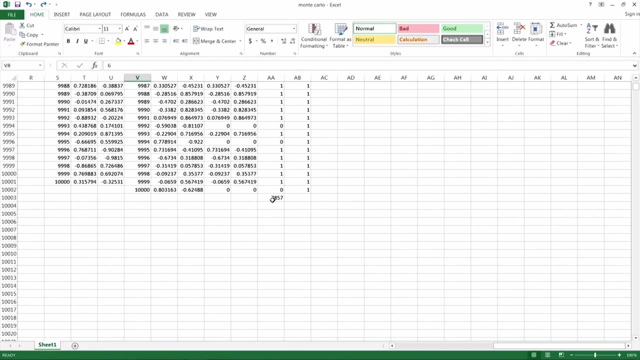 So what we can see here is that in this simulation that is done for Monte Carlo, which is, for, suppose, 10000 or more number of iterations, and when it was done for quite large number of iterations, So after doing about 10000 of iterations, what was seen was: So what, after doing 10000, 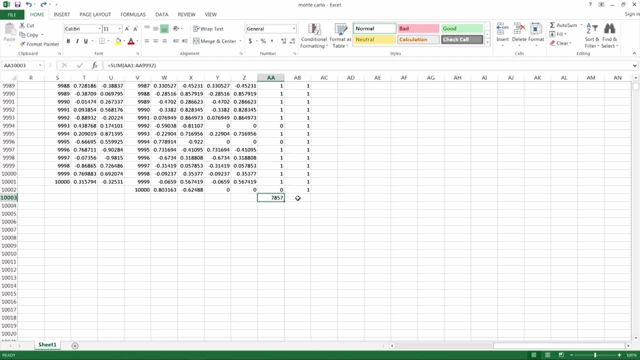 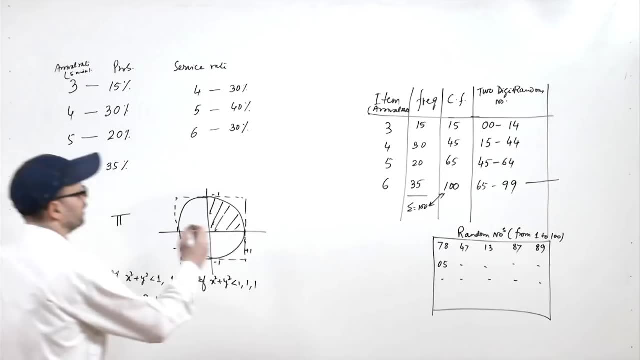 of iterations, it was seen that, out of 10000, 7857 times. this is coming in that reason, So it will be 3857 out of 10000.. Now this area of, since the area of this square is 4.. 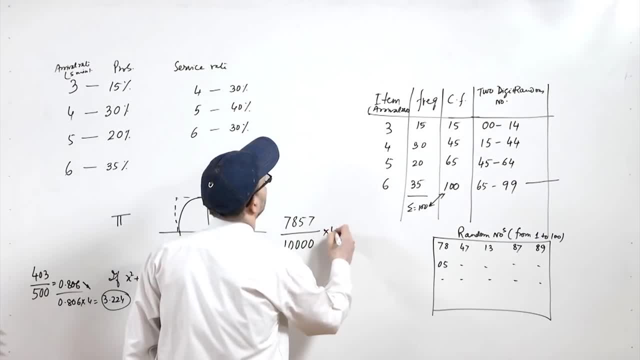 So you have to multiply it with 4.. So if you multiply it with 4 it will be p, pi. So if you would see that, it will be again 31428 by this value, So you will have 3.14. it is. 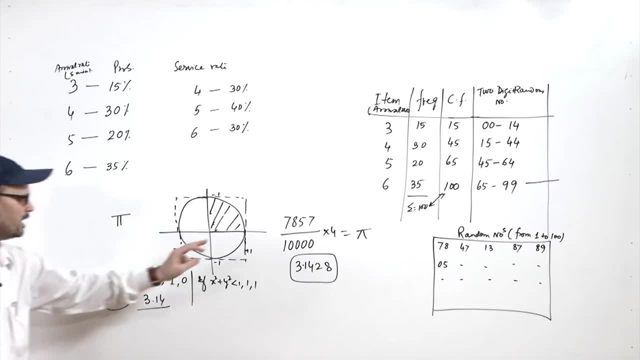 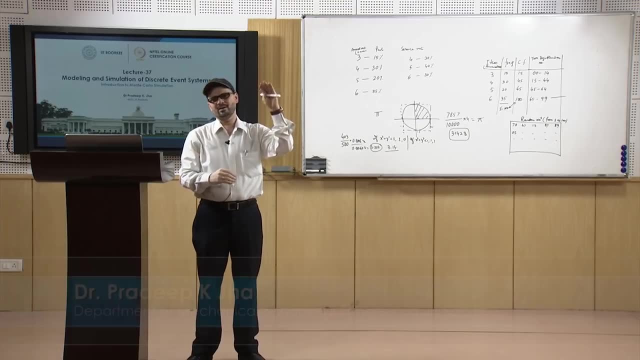 coming very much closer as this with respect to this value: So as you go on increasing that, So you have these random number streams from 100 or 500 to 10000, and if you go more and more, then in that case it is coming closer and 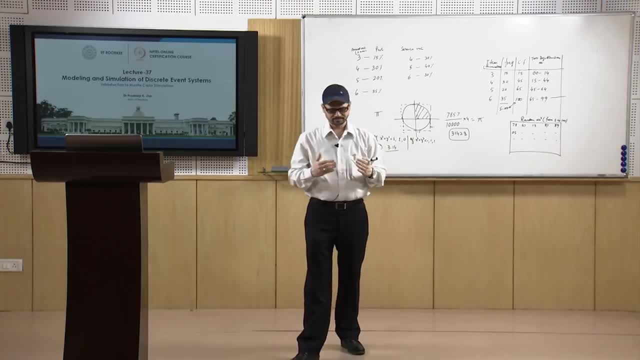 closer. So this is the concept of using the random numbers, in that if you do for the large number of iterations, you will see the average values which will be coming closer to. So that will talk about the expected value of the parameter.